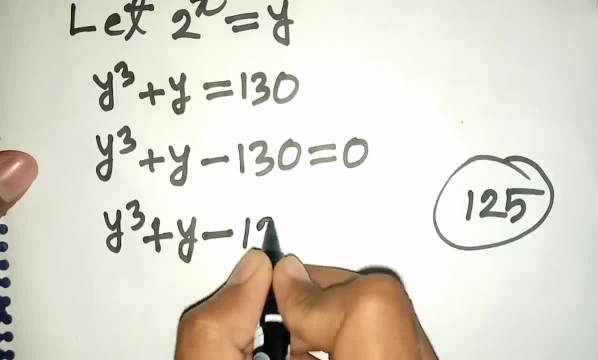 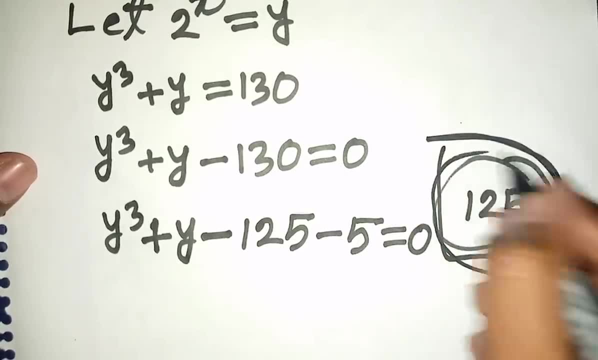 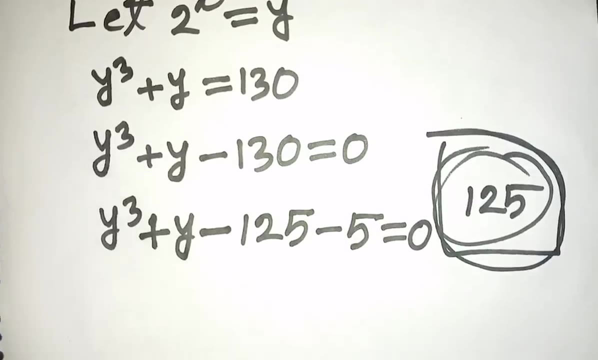 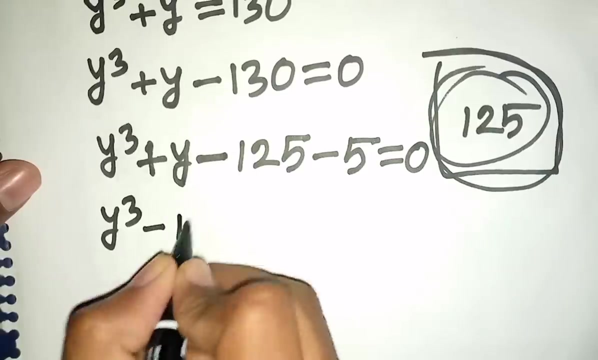 30 is same as minus 125 minus 5 is equal to 0.. Now, so minus 130 is same as minus 125, minus 5 is equal to 0.. Now we can write here: y cube, then minus 125 plus y, then y cube plus y is equal to. 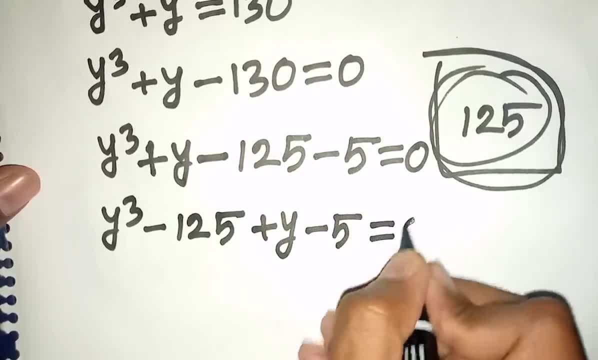 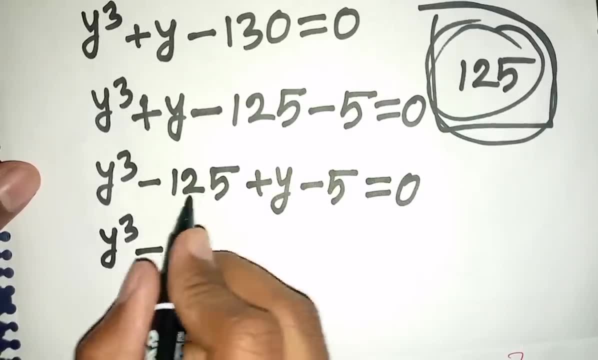 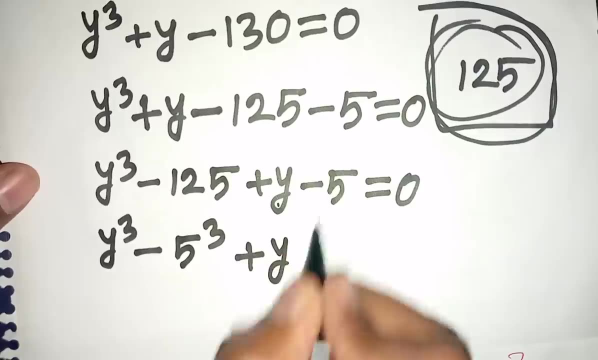 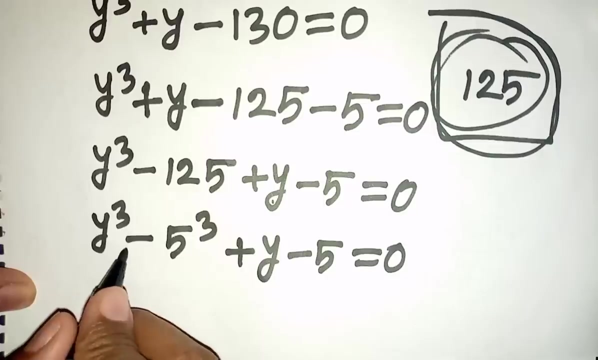 zero. Now we can write here: y cube minus 125 is same as 5 cube. then plus y minus 5 is equal to 0.. Now here we can apply the formula of a cube minus b cube. Here a is S y, b is b, So semi-preserve. 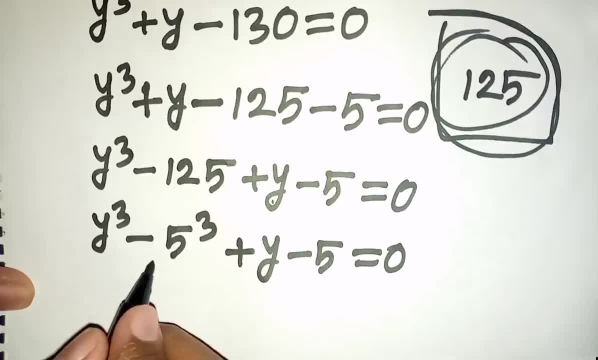 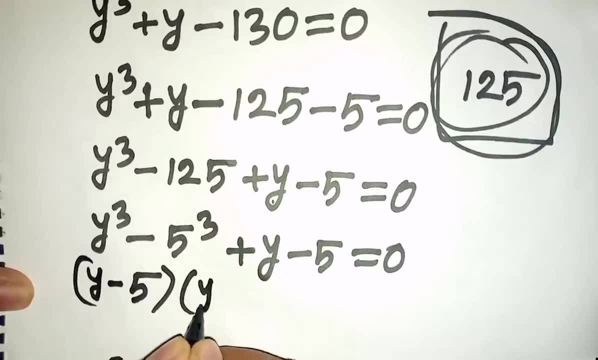 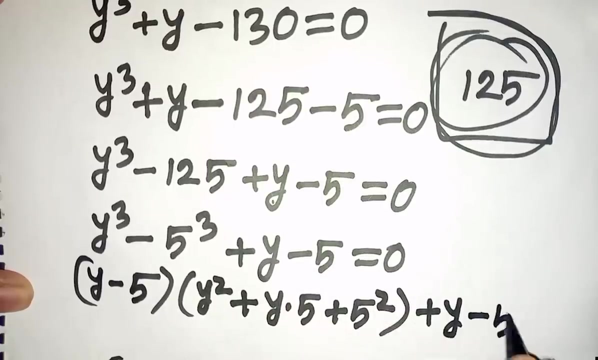 Danielle Hurley is the være. She is now going to fulfill the formula of the positive and negative y. b is s5, so according to formula we can write here: y minus 5 times y square, plus y times 5 plus 5 square, then plus y minus 5 is equal to 0.. 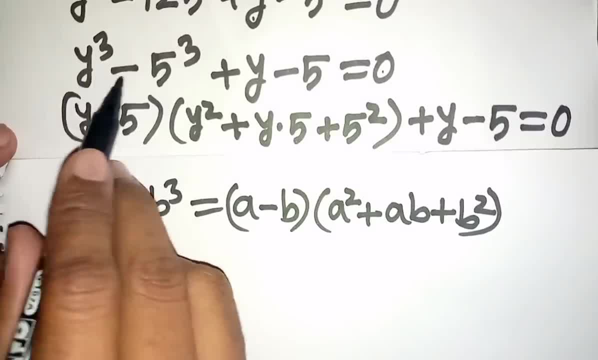 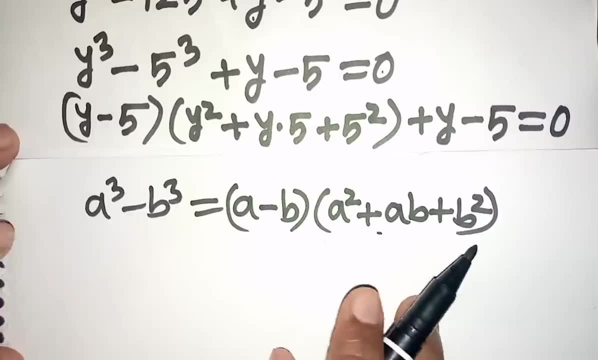 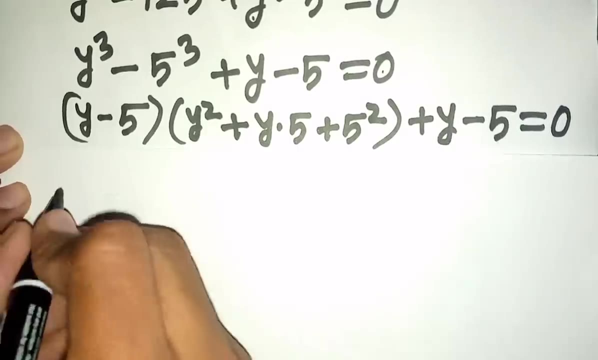 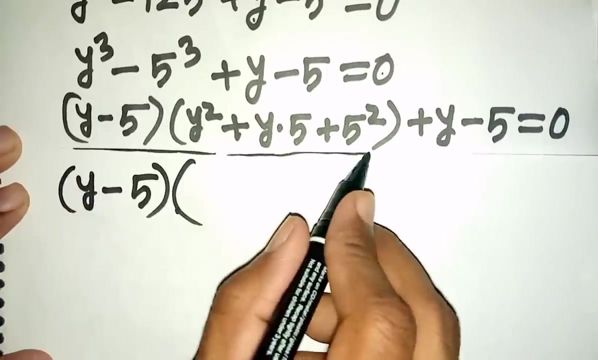 So now here we applied the formula of a cube minus b cube is equal to a minus b times a square plus a, b plus b square. so now we see y minus 5, y minus 5 is common, so bracket: y minus 5 is out of this bracket. so this divided by this, that means y square plus b. 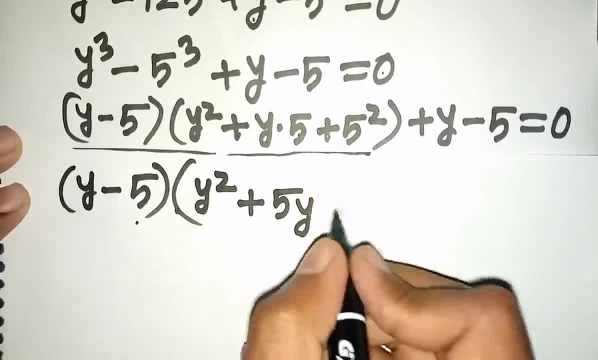 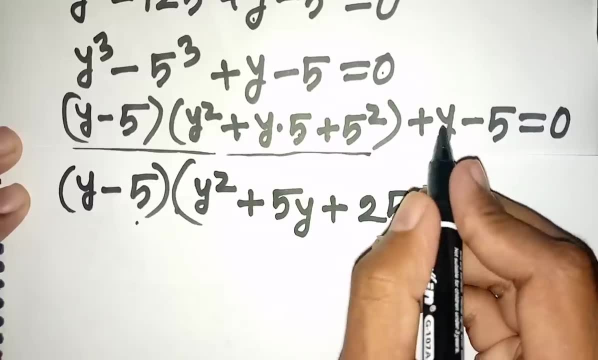 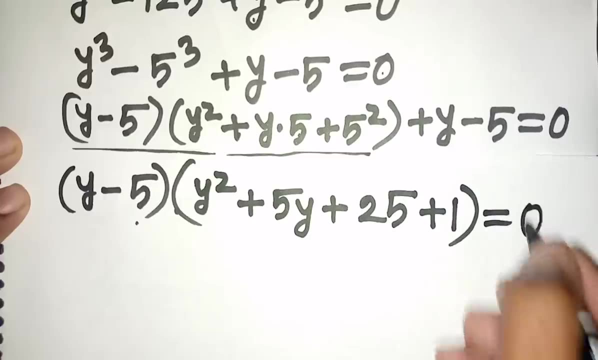 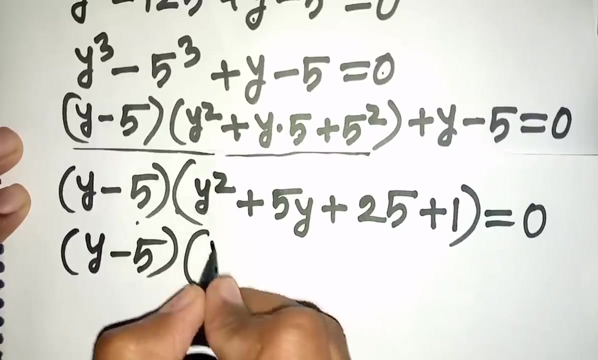 y times 5, it will be 5y plus 5. square, that means 25, then plus y minus 5, divided by y minus 5, that means 1 is equal to 0.. Now we can write here: bracket y minus 5 times y square plus 5y. 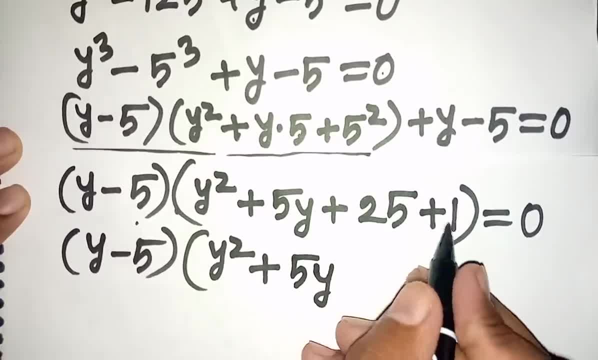 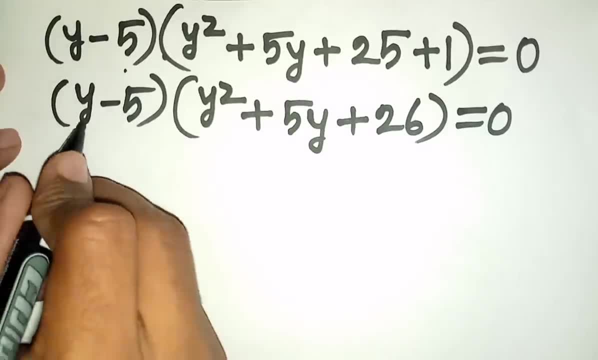 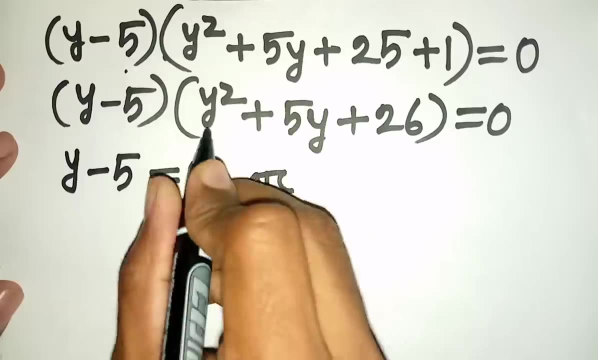 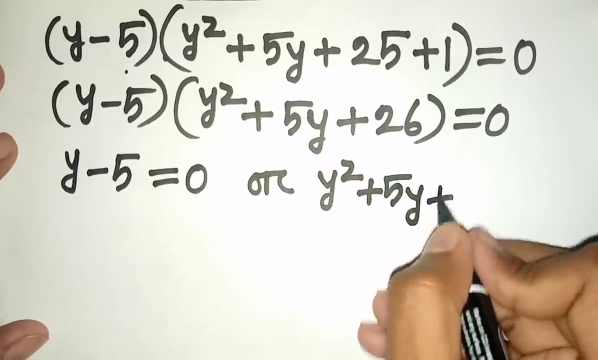 Then plus 25 plus 1, that means plus 26 is equal to 0.. Now we can write here: y minus 5 is equal to 0, or y square plus 5y plus 26 is equal to 0.. 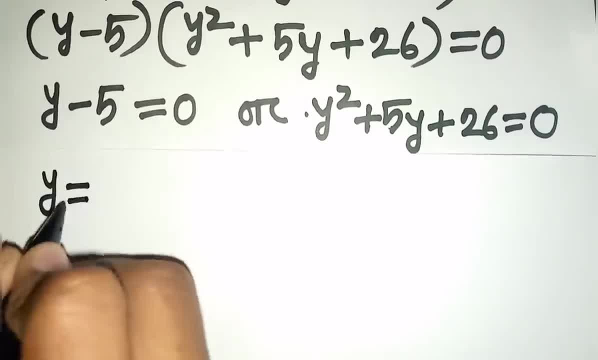 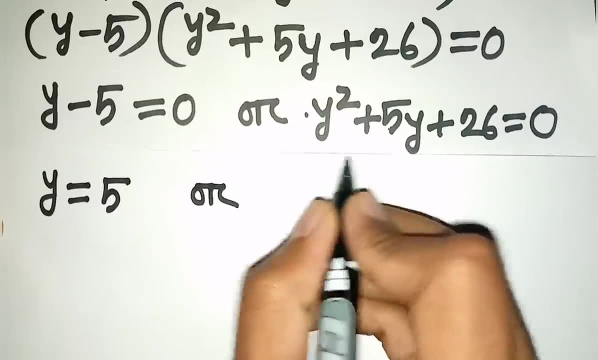 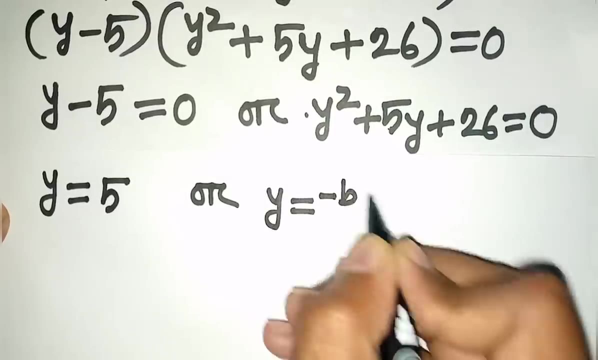 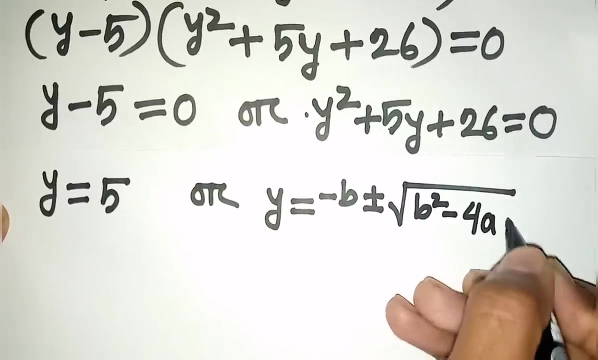 So now we can write here: y is equal to minus 5. take to the right side, so this will be plus 5. or here we can apply quadratic formula, so we can write here: y is equal to minus b, plus or minus a square root of b square minus 4ac divided by 2a. 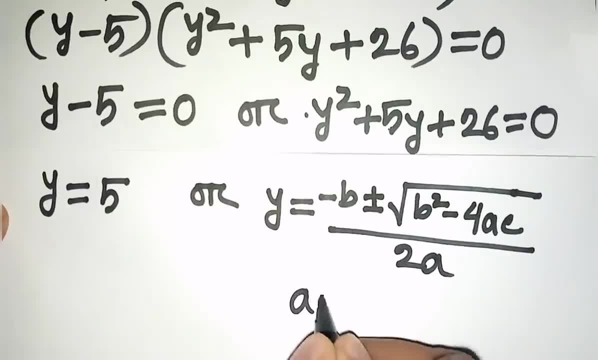 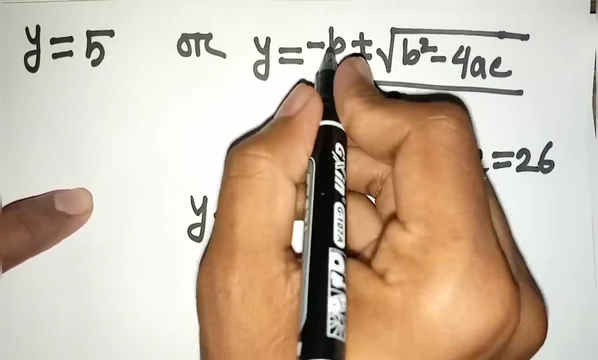 Now here: a is s1, b is s5, c is s26.. So we can write here: y is equal to minus b, that means 5.. Now if we calculate the brings at the straight path, then we will see y as 0.. 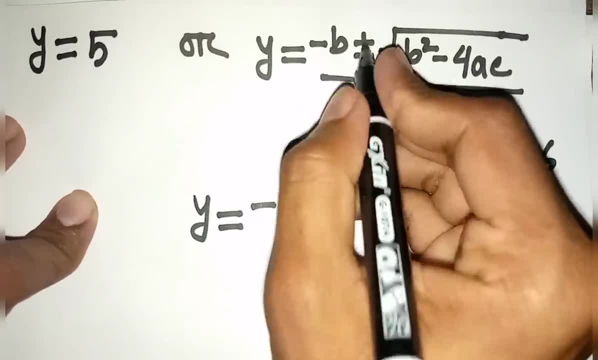 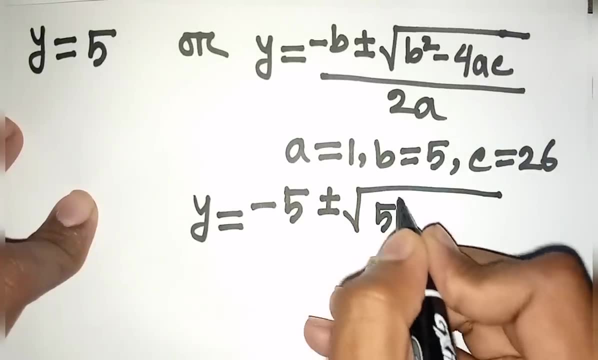 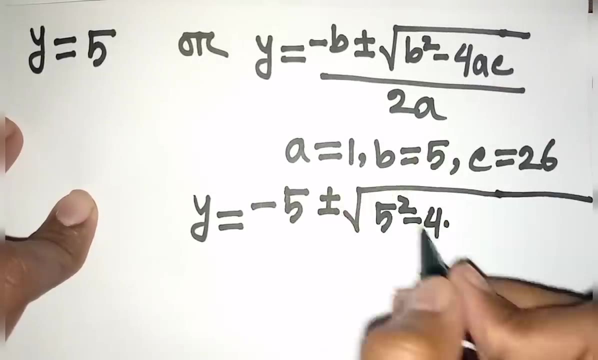 So that will be minus b, and b is also equal to b. So y equal to y, minus b, plus or minus 돈 hs3呢 a square root of b square. that means 5 square minus 4 times a. that means 1 times c. that means: 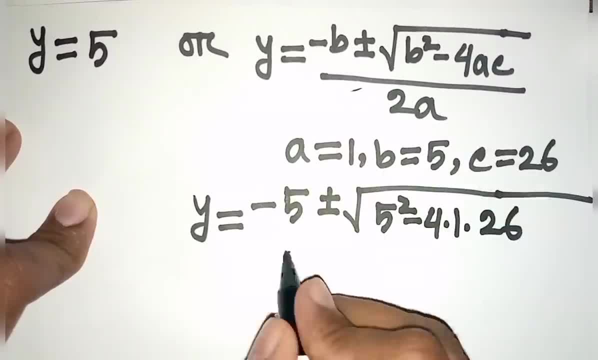 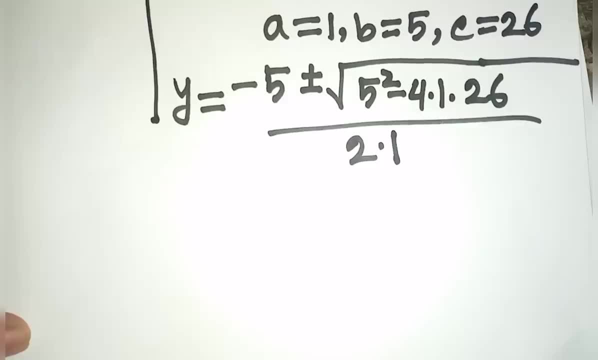 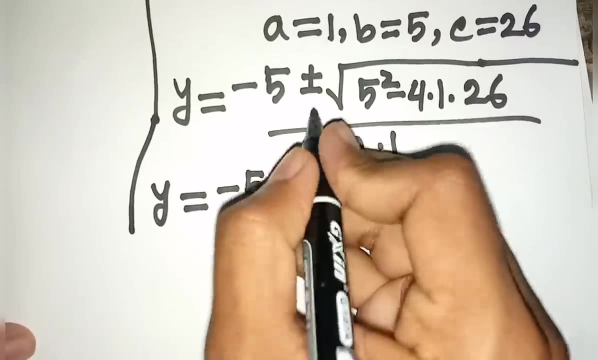 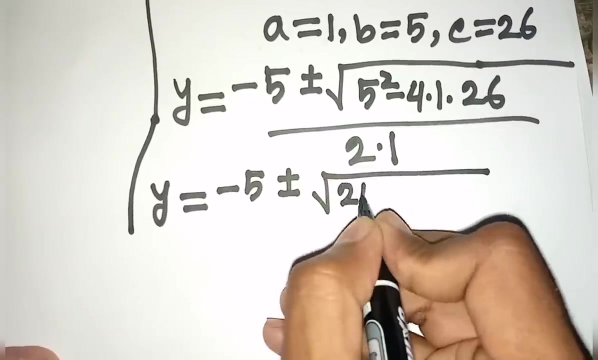 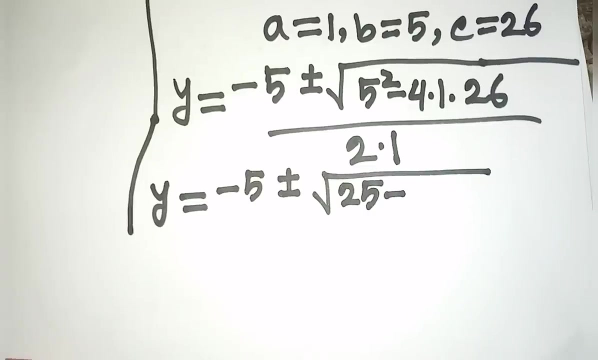 26 divided by 2 times a. that means 1.. Now we can write here: y is equal to minus 5, plus or minus a square root of 5 square. that means 25 minus 4 times 1 times 26.. That means 104 divided by 2 times 1, that means 2.. Now we can write here: y is equal to minus 5. 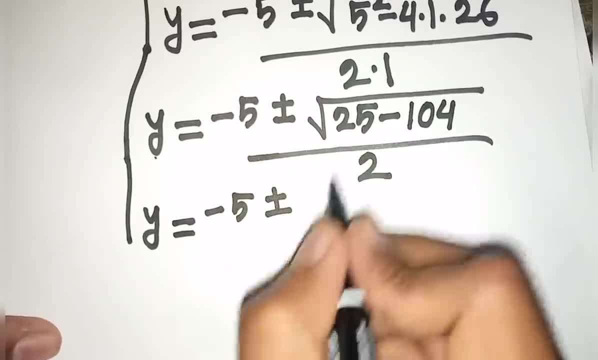 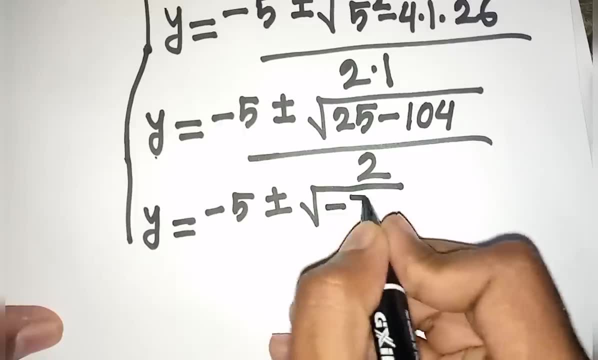 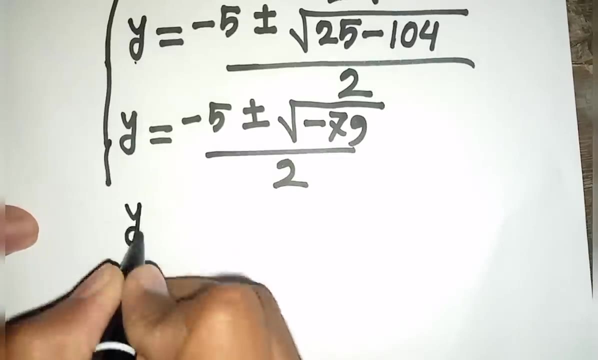 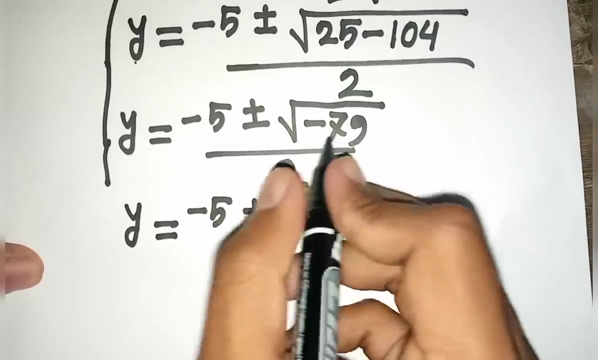 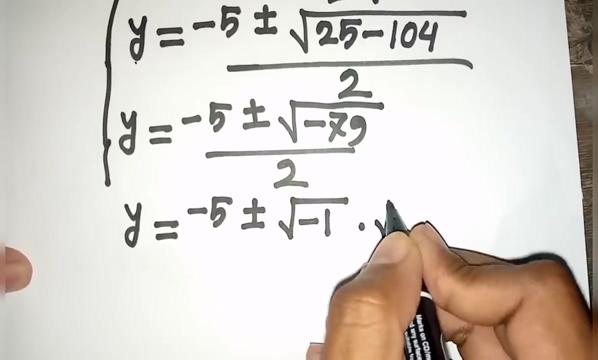 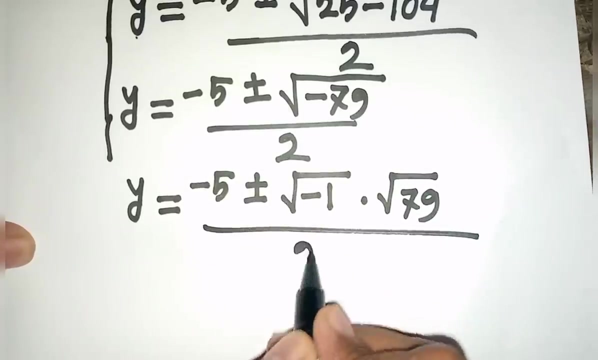 plus or minus a square root of 25 minus 104. that means minus 79 divided by 2.. Now, now we can write here: y is equal to minus 5 plus or minus. a square root of minus 79 is same as a square root of minus 1 times a square root of 79.. Now, divided by 2.. Now we can write here: 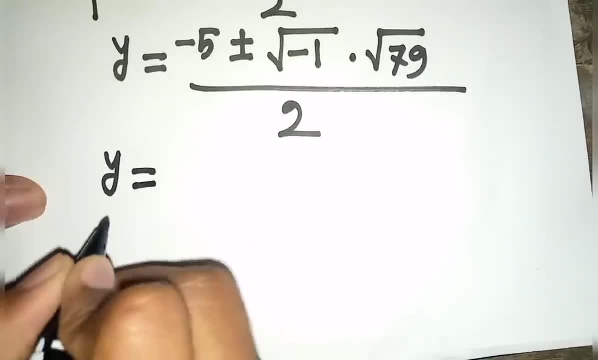 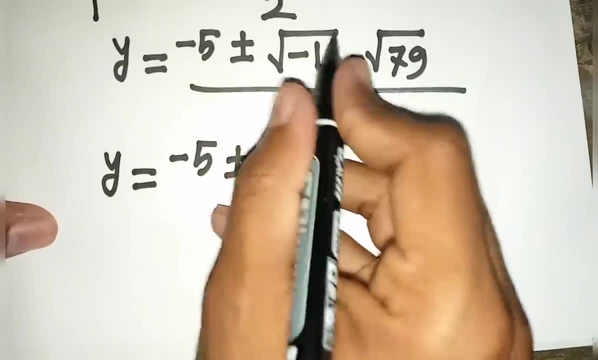 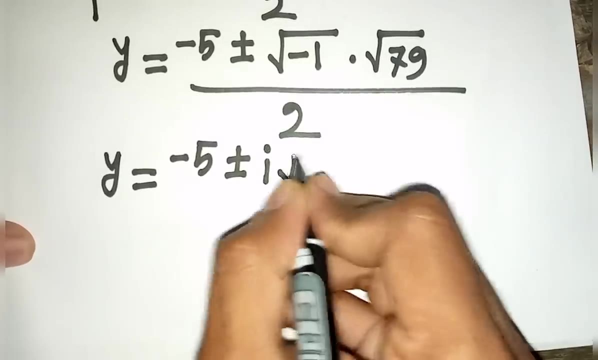 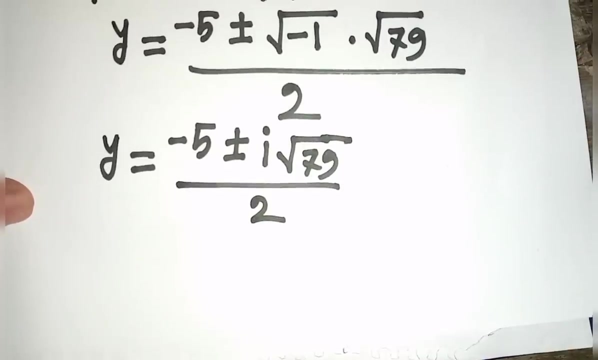 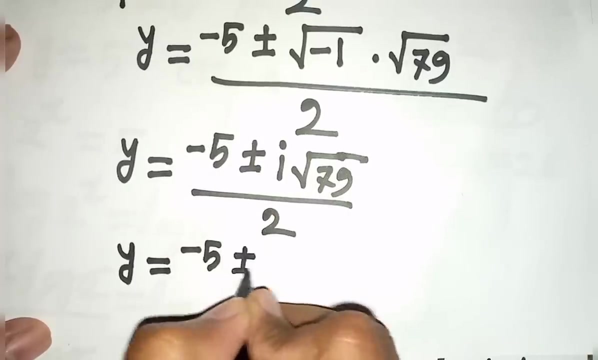 y is equal to minus 5 plus or minus, a square root of minus 1. that means imaginary, then, a square root of 79, a square root of 79 divided by 2.. Now we can write here: y is equal to minus 5, plus or minus. 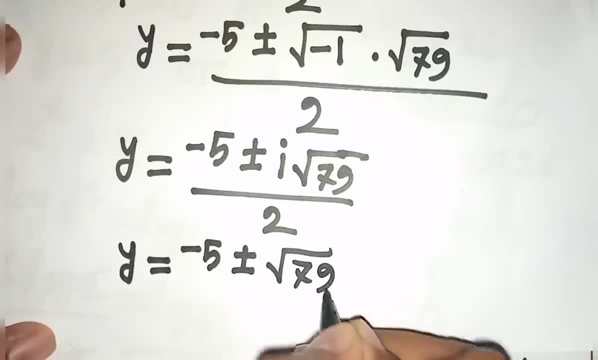 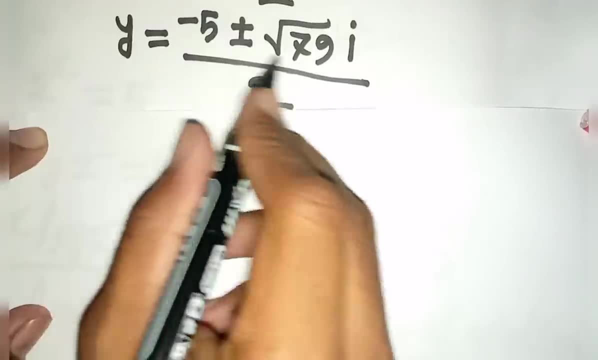 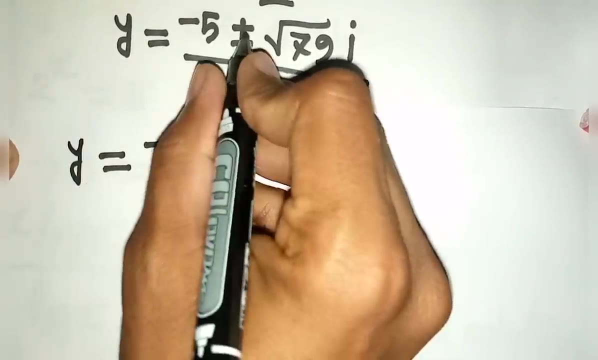 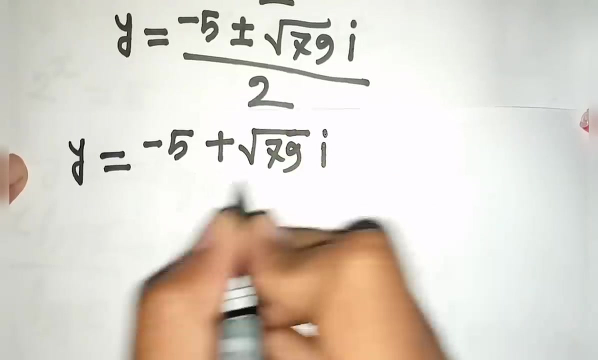 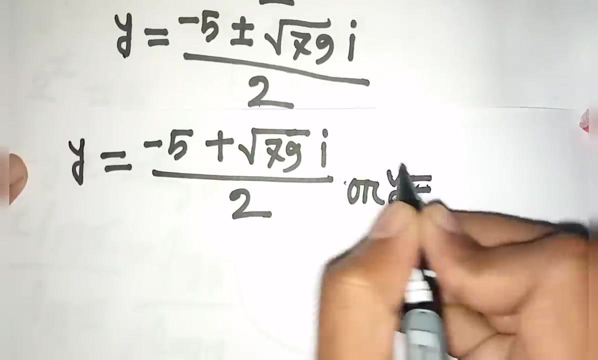 a square root of 79 imaginary divided by 2.. So now we see here two cases, so we can write here: y is equal to minus 5 plus or minus a square root of 79 imaginary divided by 2, or y is equal to minus 5 plus or minus a square root of 79 imaginary divided by 2.. So y is equal to: 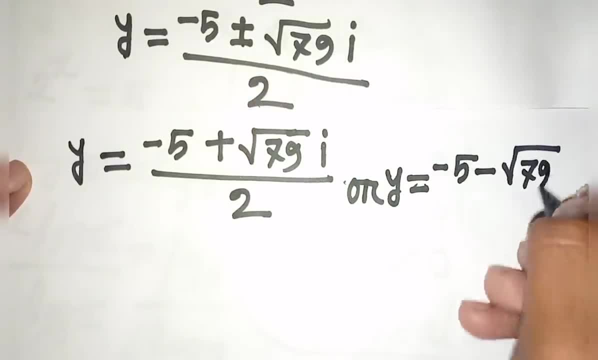 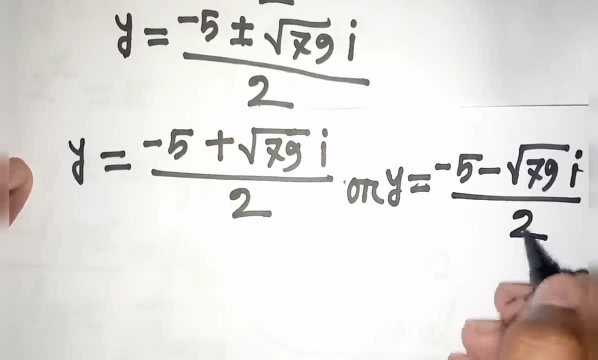 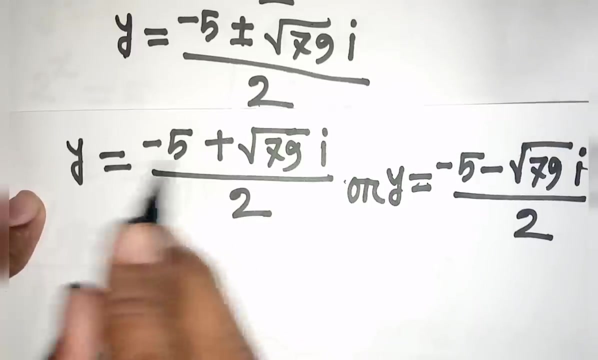 minus 5 plus or minus a square root of 79 imaginary divided by 2. or y is equal to minus 5 plus or minus a square root of 79 imaginary divided by 2.. So y is equal to minus 5 minus a square root of 79 imaginary divided by 2.. This 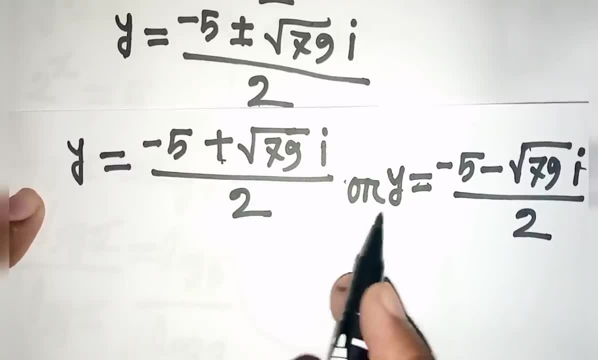 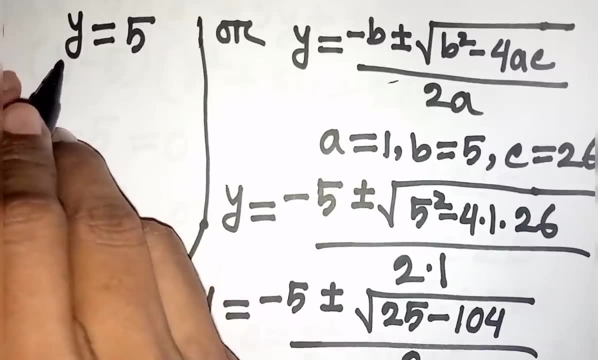 value and this value are not accepted Because these are imaginary values. so our final, the final value of y will be: y is equal to 5.. But remember, y that means let 2 power. x is substituted with c. Now. now let us write: y is equal to i, for x is l, which we have now removed from the 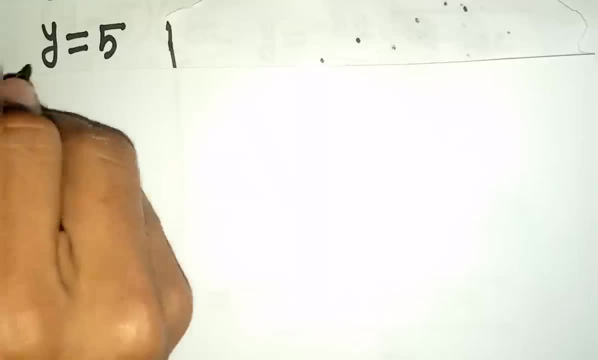 equation. Now let us see again where is 1. it is not evil c, but this is y xi, where this y xi implies: by y So y, that means 2 power x So y, that means 2 power x is equal to 5.. Now we take log. 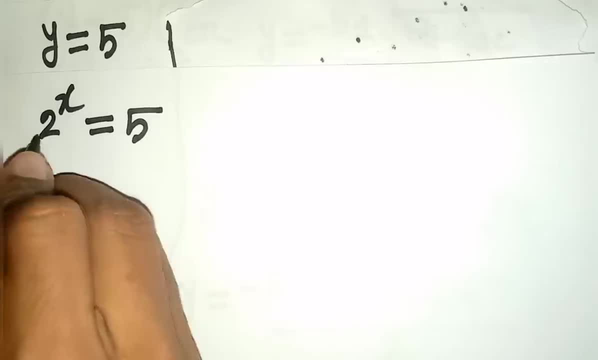 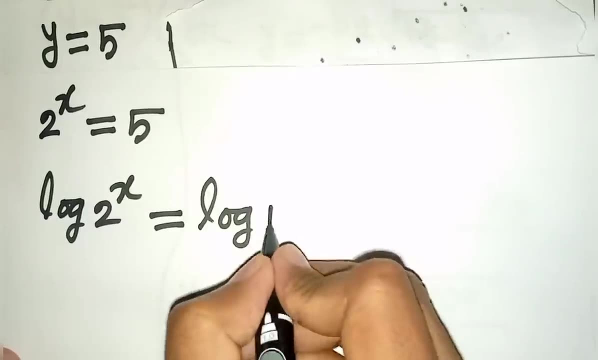 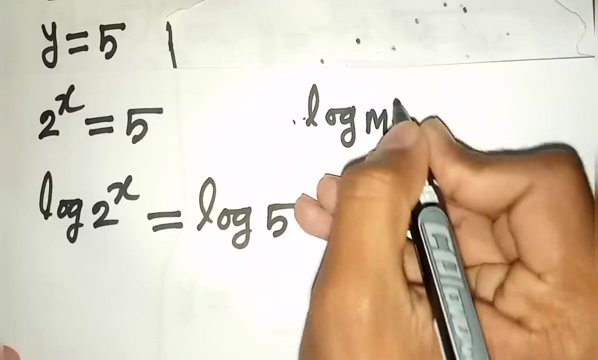 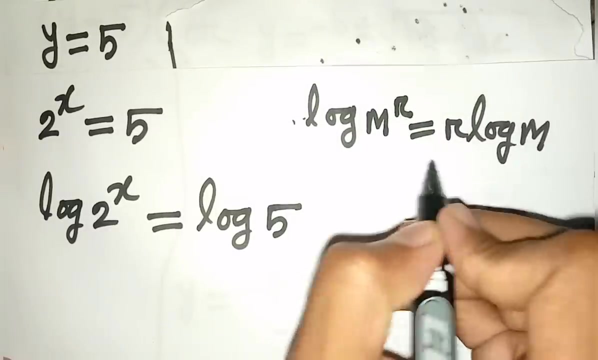 both sides. So we can write here: log 2, power x is equal to log 5.. Now here we can apply this formula: log m, power r is equal to r log m. That means this power move to here. So according to: 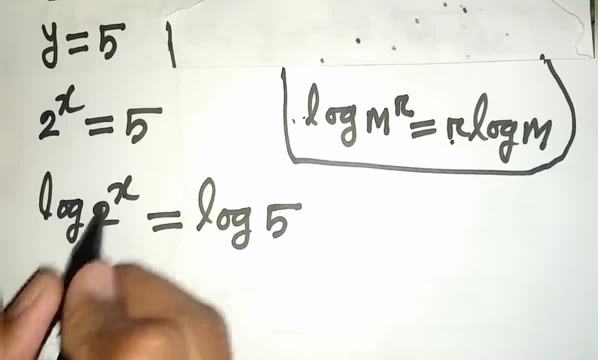 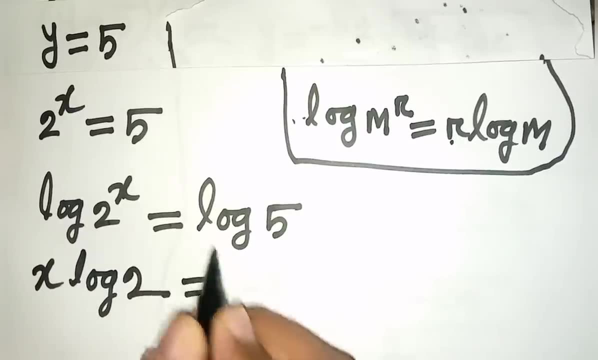 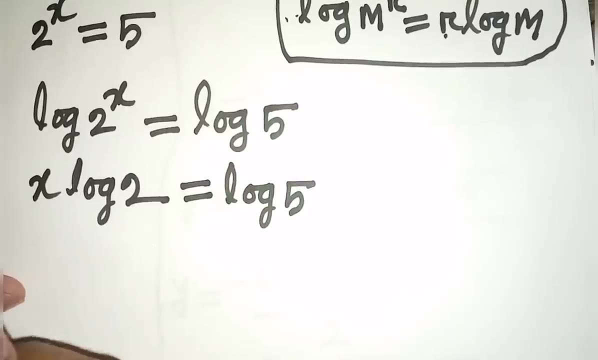 this formula we can write here, this power move to here. So x log 2 is equal to log 5.. Now we can write here: x log 2 is equal to log 5.. We need the value of x, So we divided by log 2 both sides. So divided by log 2, divided by log. 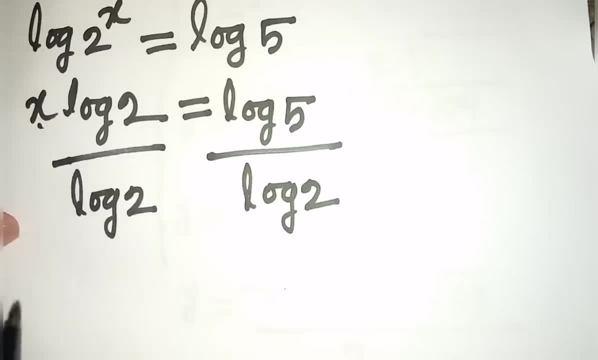 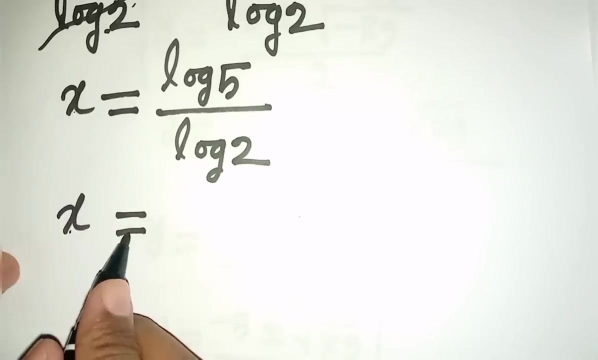 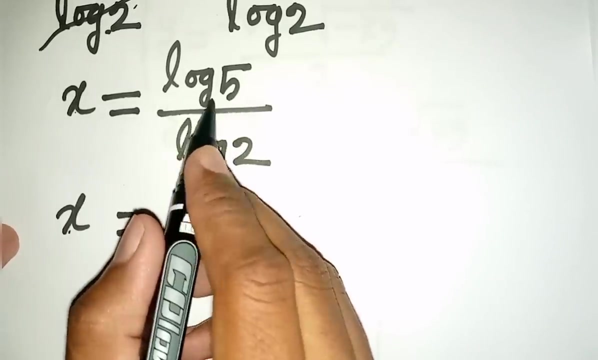 2. Now we see this log 2 will be cancelled. So here x is equal to log 5 divided by log 2.. Now we can write: here x is equal to: here We can use calculator. So log 5, that means the. 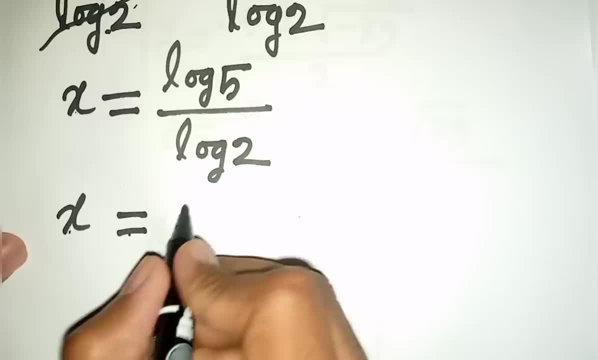 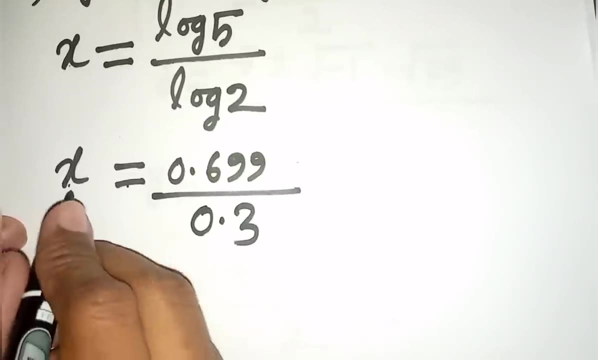 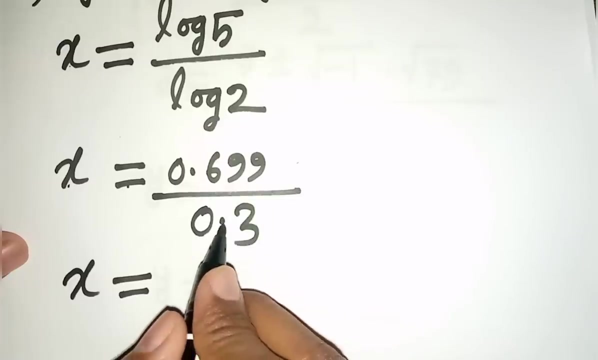 approximate value of log 5 is 0.699 divided by log 2.. That means the approximate value of log 2 is 0.3.. Now we can write here: x is equal to 0.699 divided by 0.3. That means 2.33.. So this is the value. 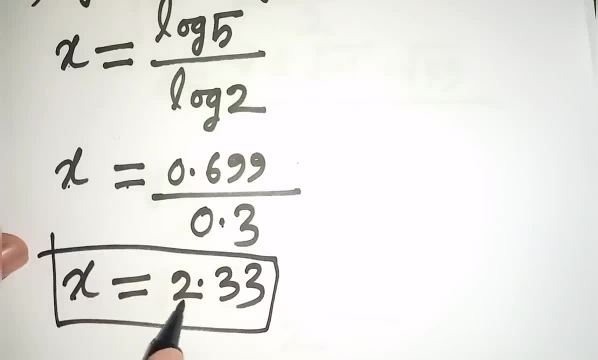 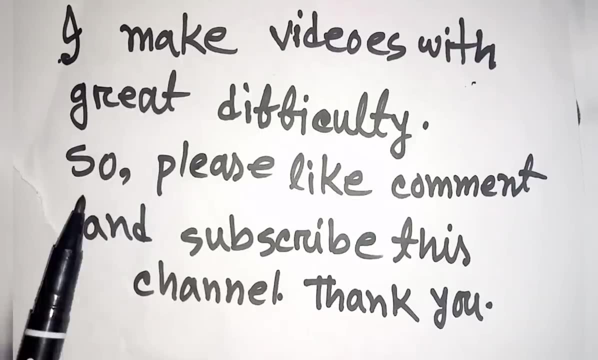 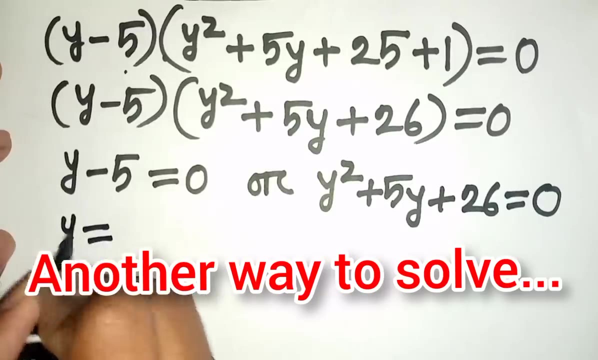 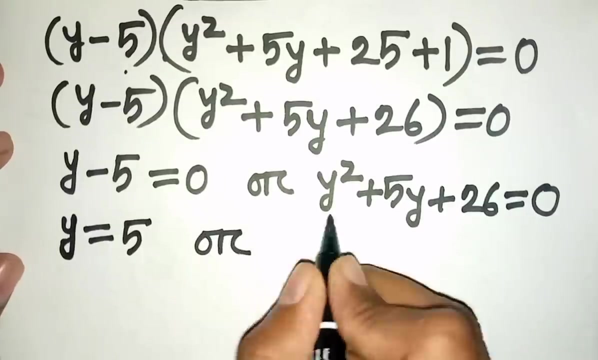 of x. So our final answer: x is equal to 2.33.. I make videos with great difficulty, So please like, comment and subscribe the channel. Thank you. Here y is equal to minus 5.. Take to the right side. So this will be plus 5, or here we can. 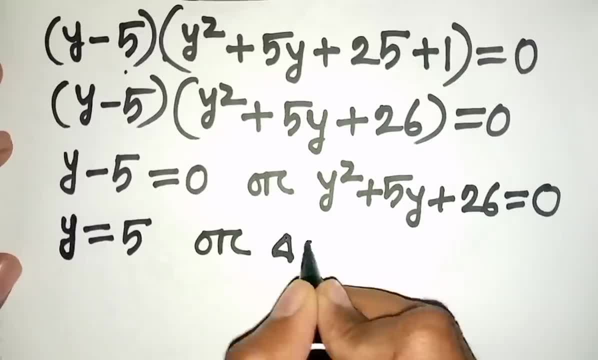 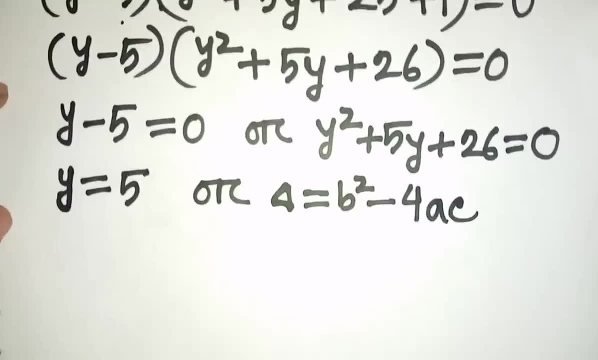 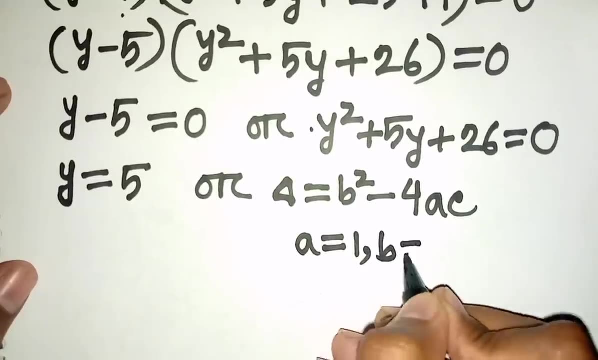 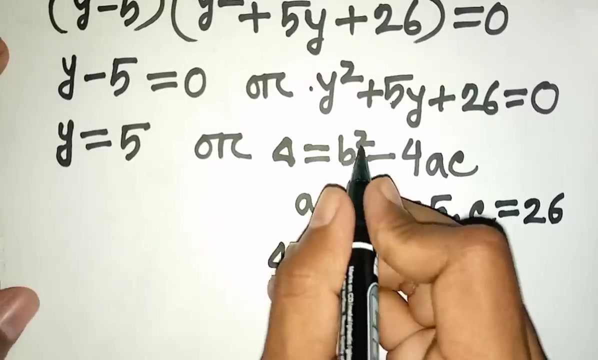 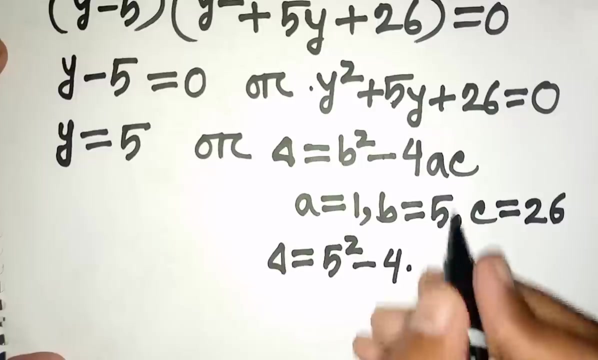 apply discriminate formula: Delta is equal to b square minus 4 ac. Now here a is s on, b is s 5. So we can write here: delta is equal to b square. that means 5 square minus 4 times a. that means on times c, that means 26.. 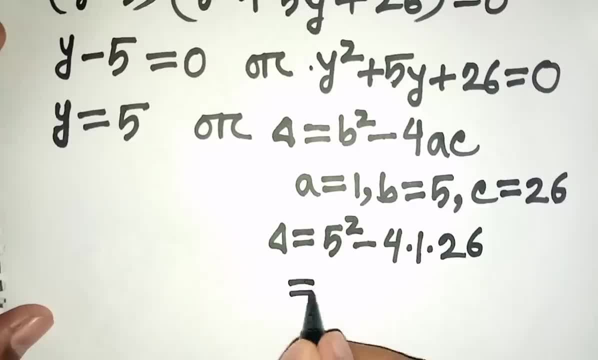 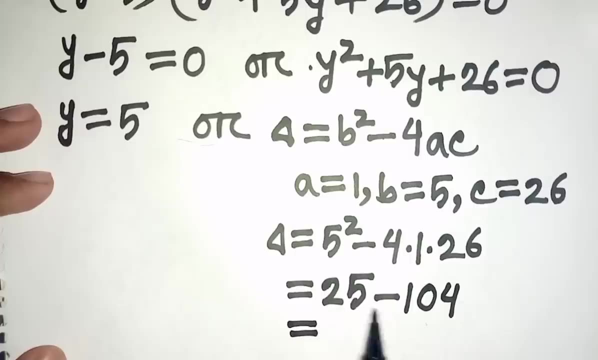 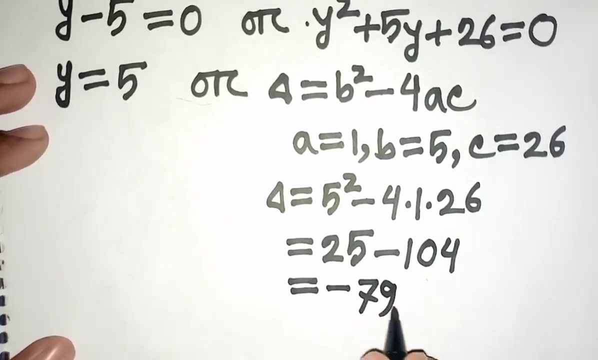 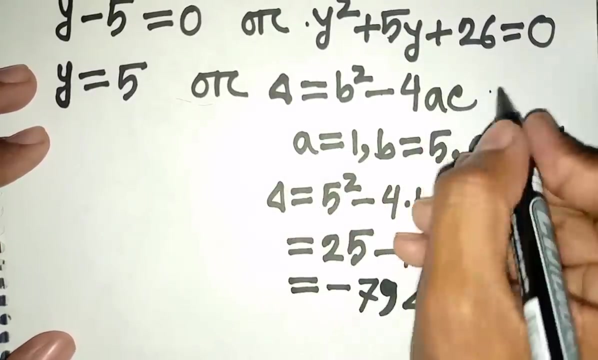 Now we can write here: 5 square, that means 25.. minus 4 times 1 times 26, that means 104. now is equal to 25 minus 104, that means minus 79.. So minus 79 minus 79 is less than 0. so b square minus 4 ac is less than 0.. 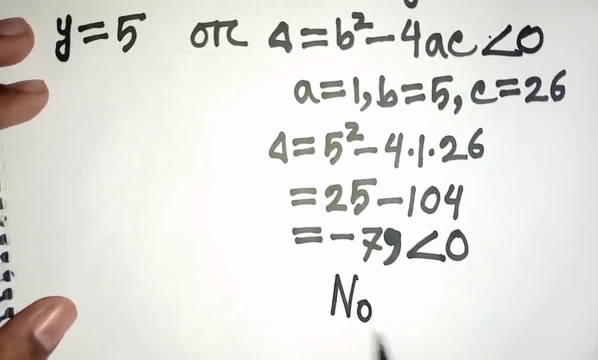 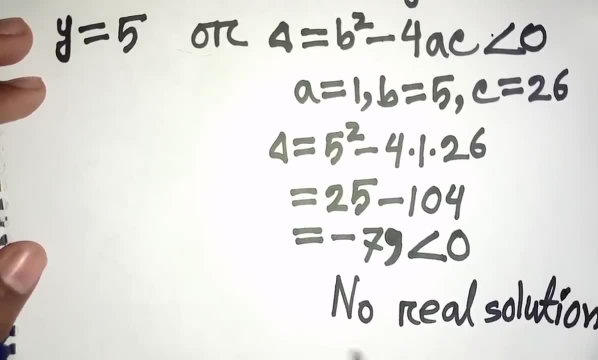 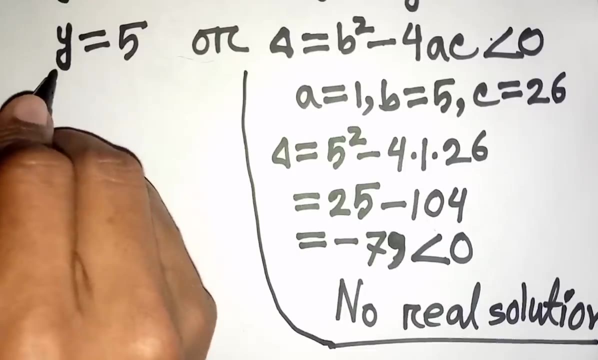 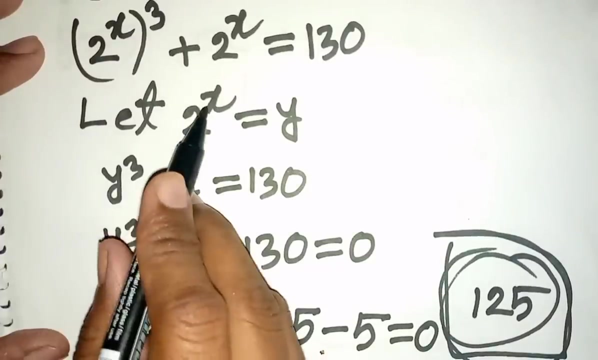 So here no real solution. no real solution. solution: minus 79 is less than 0, so here no real solution. but here y is equal to 5.. Now y that means, remember, let 2 power x is substituted by y, so y that means 2 power x. 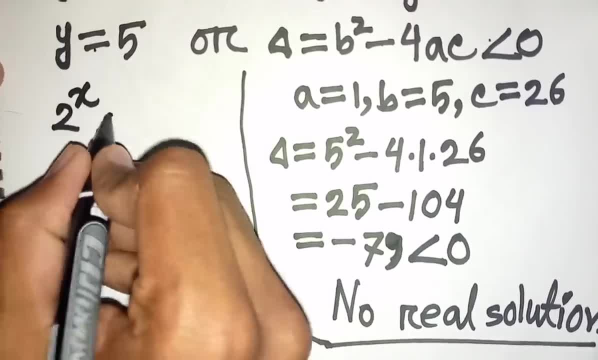 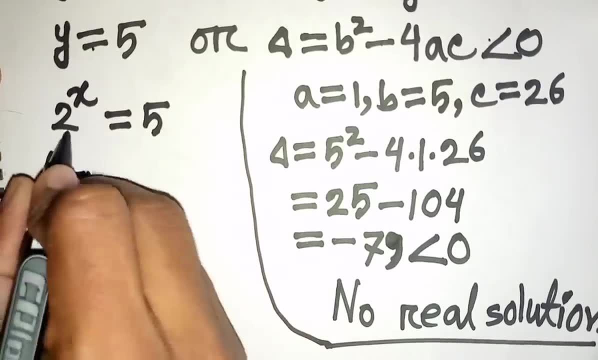 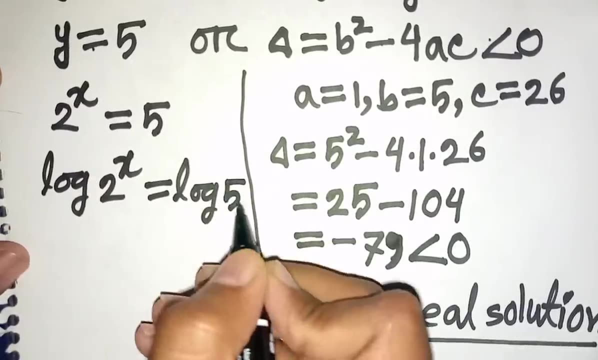 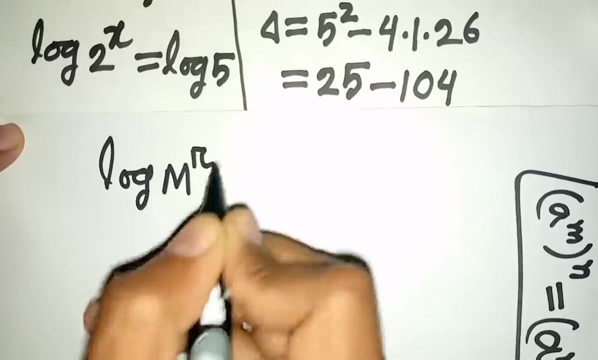 So y, that means 2 power x is equal to 5.. Now we take log both sides. so log 2 power x is equal to log 5.. Now here we can apply this formula: log m power r is equal to r log m that.